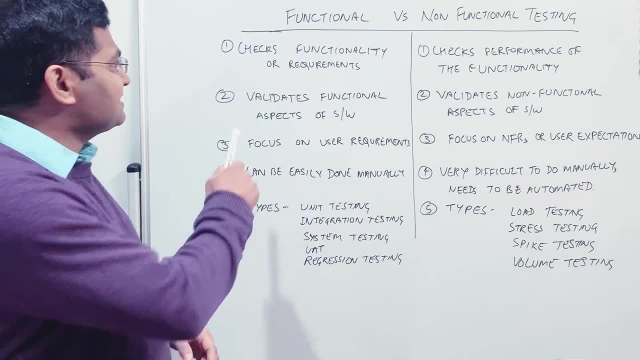 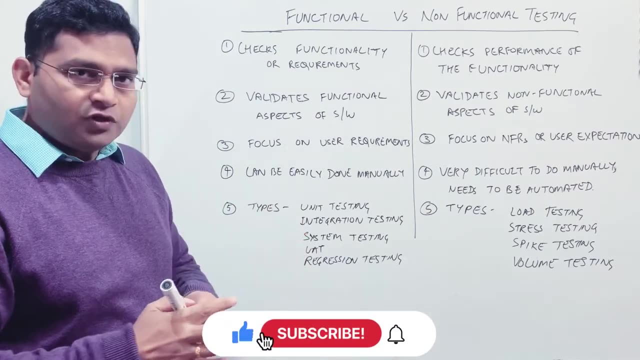 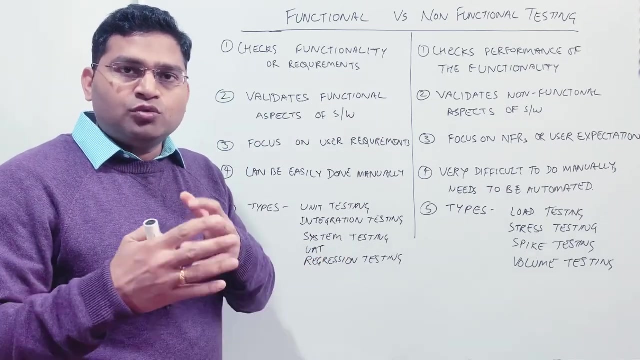 point here. So what functional testing does, is it checks the functionality or the requirements? So basically, when we say functionality or the requirements, so requirements are being given by the customer. So if say, for example, you are an organization or you are working within a team, 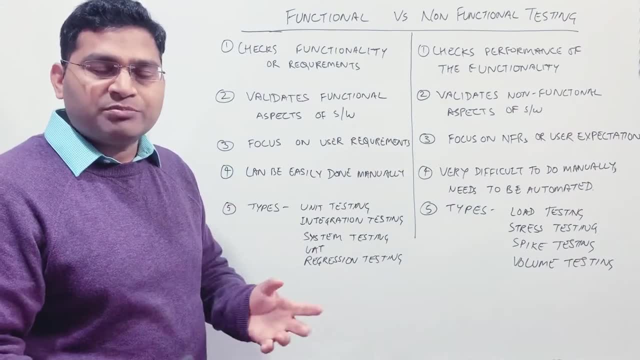 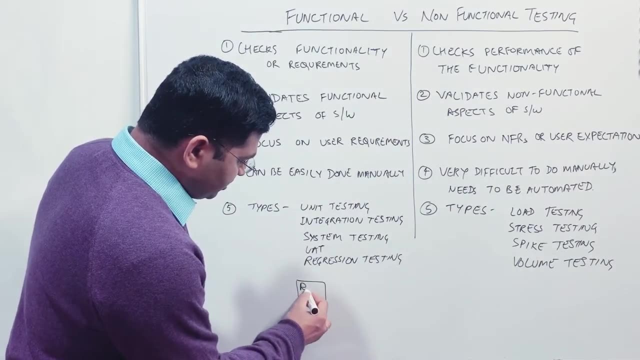 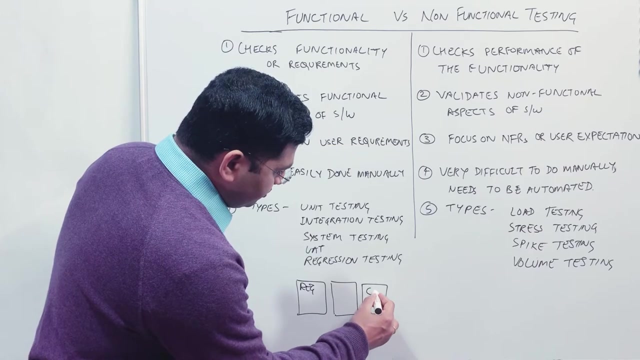 or you are a customer who wants some website or e-commerce website to be developed So that customer will give you the requirement, and the requirement could be the registration, you know, adding items, checkout. Okay, so checkout could be one payment. So, on the high. 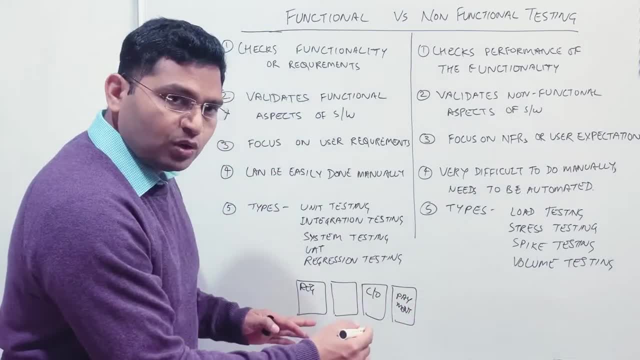 level. these could be some of the high level requirements. Now, when you are verifying these requirements, you should be able to check the functionality or the requirements. So, when you are verifying the functionality or the requirements, you should be able to check the functionality or the. 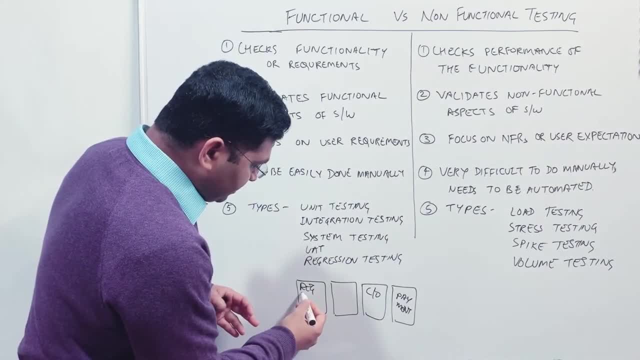 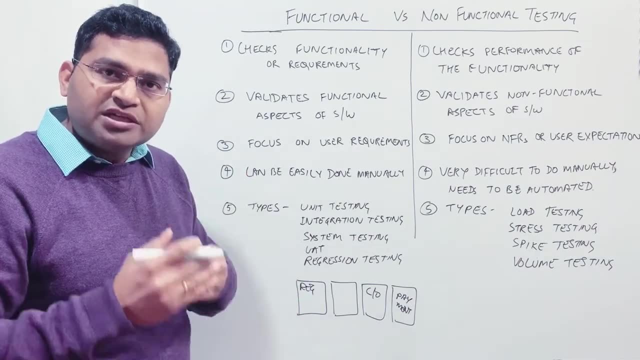 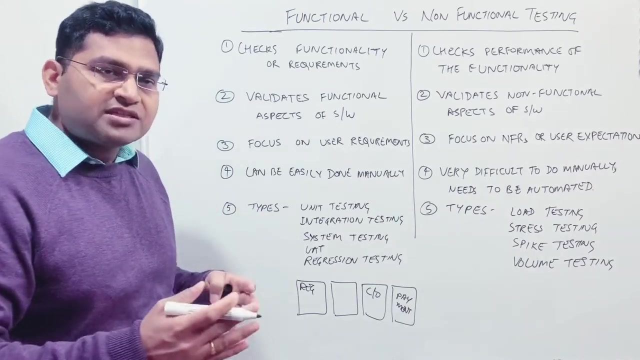 functional verification. Say, for example, as a tester I'll click on register link, I'll provide all my user details and then click on register button, And if the registration is successful and I am redirected to the dashboard page, then that sort of testing is the functional testing. or 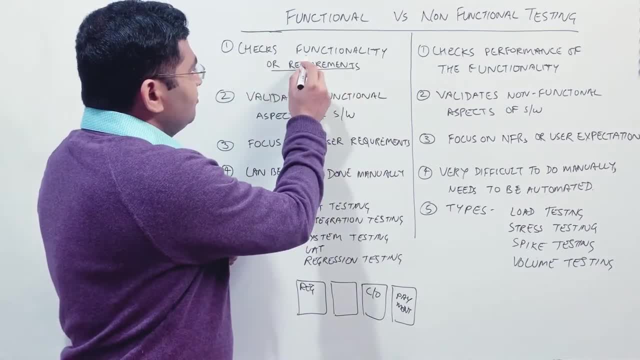 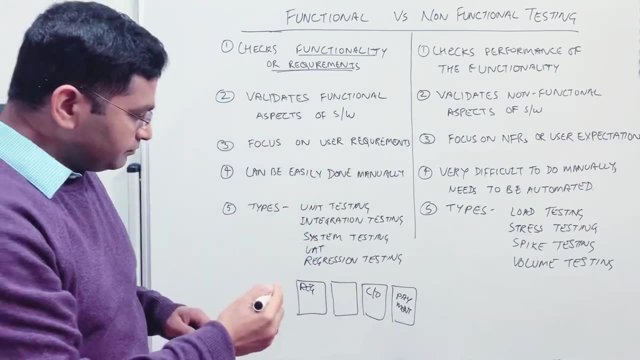 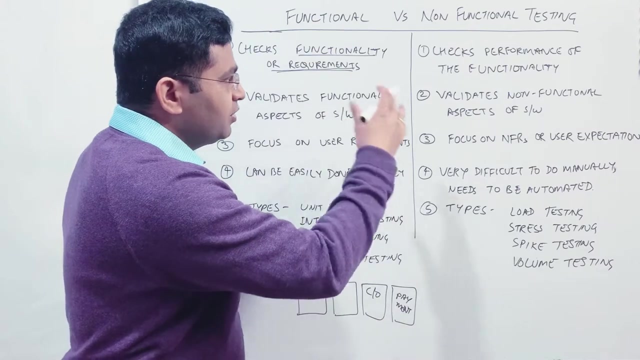 verifying the functional requirements. Okay, so verifying the functionality or the requirement is the functional testing. So when you are verifying the functionality or the requirements, you should be familiar with all these requirements. you should also be familiar with the functional testing. So now when we talk about the functional testing, then the non-functional testing verifies the. 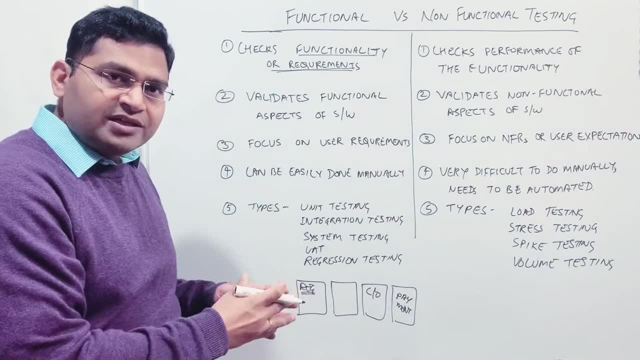 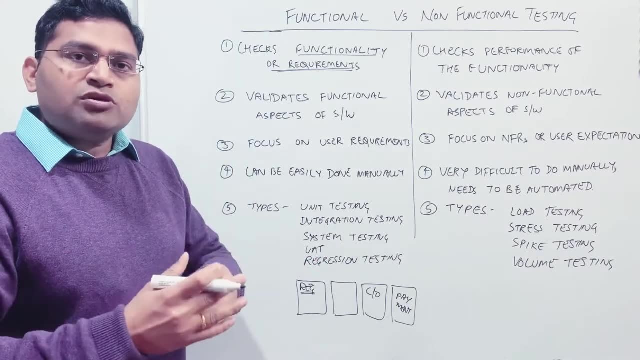 non-functional aspect or the performance of that particular functionality. So now say, for example, registration for the functional testing. I'm just concerned about whether the registration is happening successfully or not. When we talk about the non-functional testing, I'm concerned how much time it takes for a user or if you want to be a beta test or have 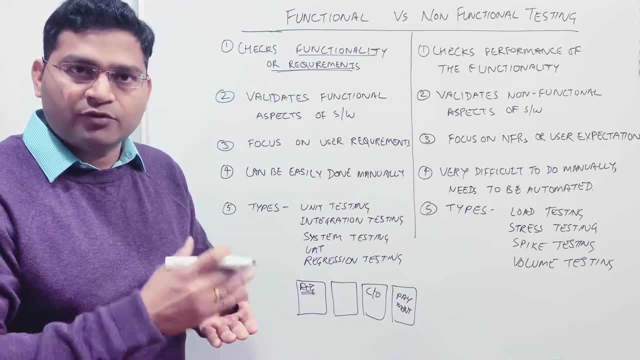 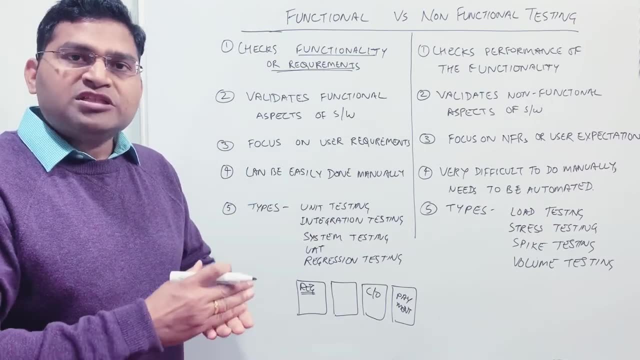 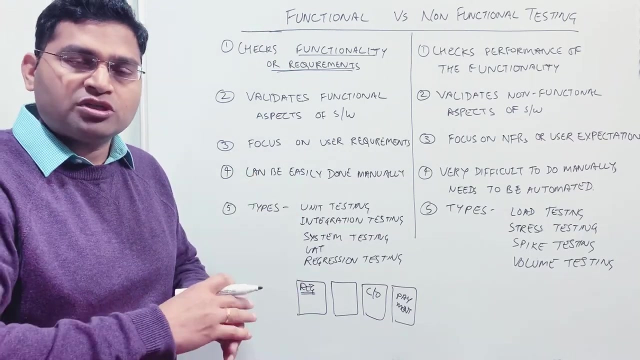 user to register. so once he clicks on, once he fills all the information or all the data into the registration form and clicks on register button, how much time it takes for the user from clicking the register button to be redirected to the dashboard page. so, because that there is a 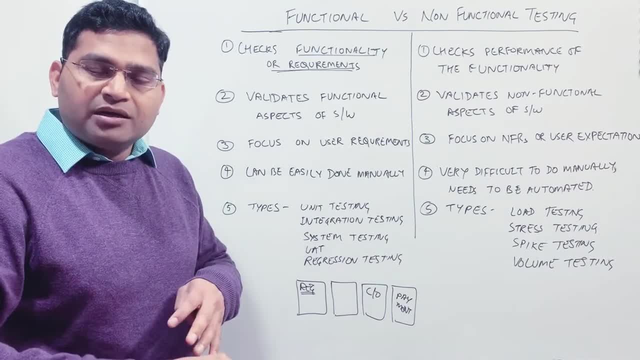 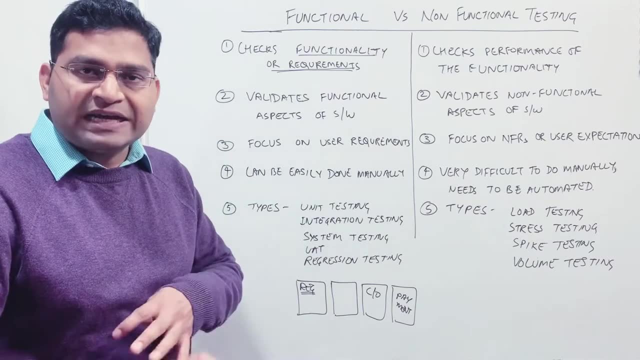 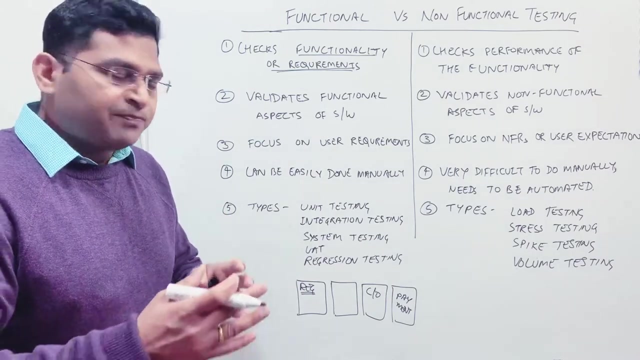 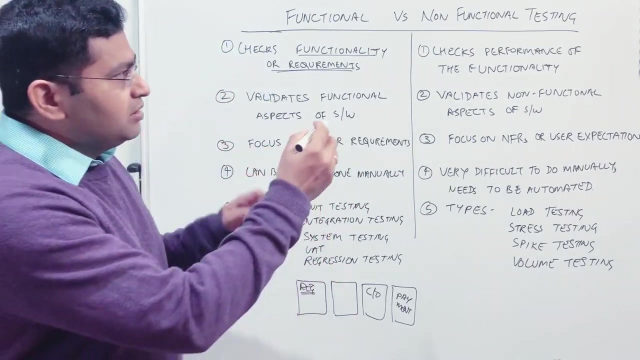 processing that happens at the server end in the back background. after user clicks on registration button, the user gets registered or entries are added into the database, is given a session id or the user id and then redirected to the dashboard page. so if you are verifying that performance of the functionality that you are testing manually, then that is non-functional. 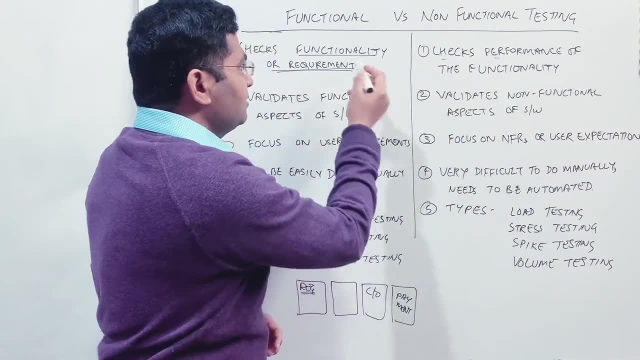 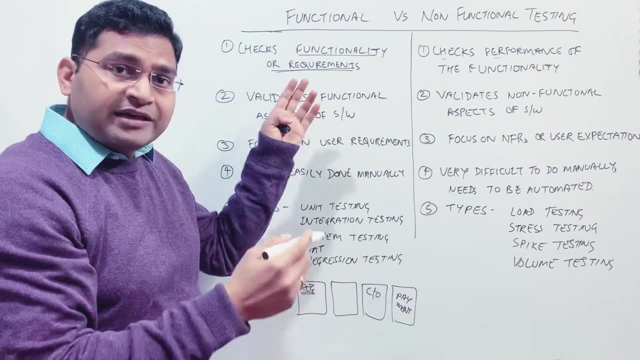 testing. so non-functional testing checks performance of the functionality. so we have taken example, or taken an example, of the registration for the functional testing. so we have taken an example of the registration for the functional testing and similar example for the non-functional testing, right? so what you will verify in the 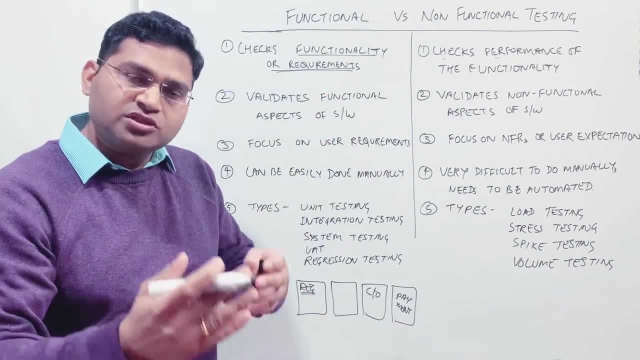 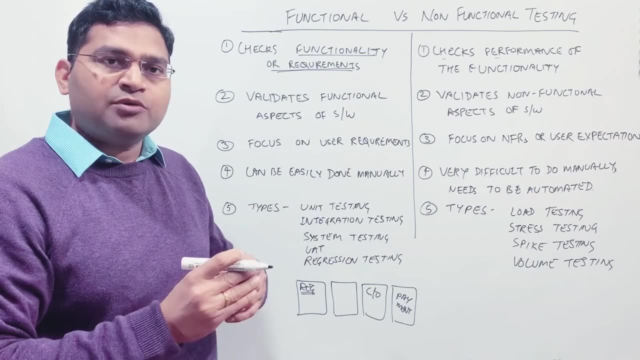 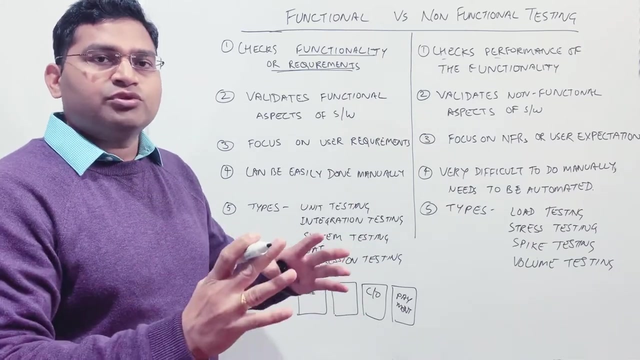 non-functional testing for the same functionality. so you'll verify the response time. you'll verify how the system behaves, or what is the you know response time or reliability, when there are multiple users accessing the same functionality or there is a lot many users accessing the application, right? so that is basically checking the performance of the functionality. 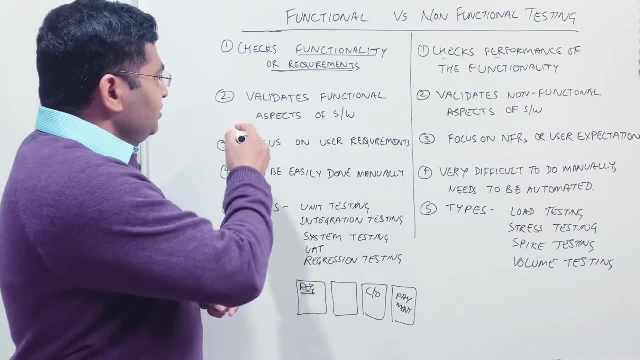 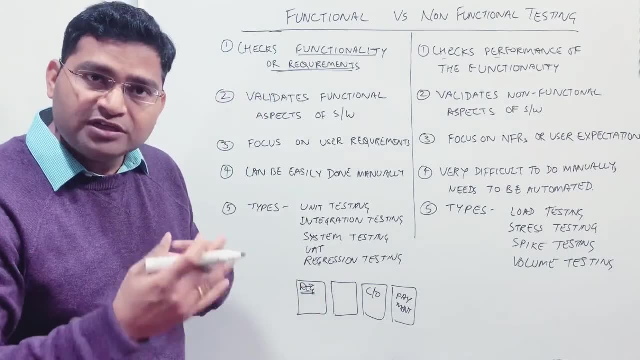 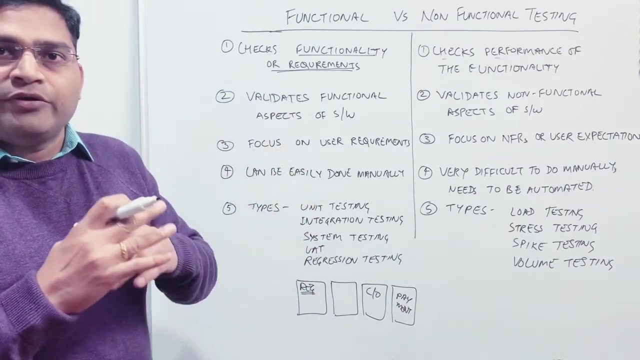 so that is non-functional testing. second point is: validate the functional aspect of the software. so functional aspect, as we see, registration. so when you are, you know manually filling, clicking on the registration link, filling out the data and registering. that's the functional aspect of it. non-functional is, as we have covered in the first part, non-functional. 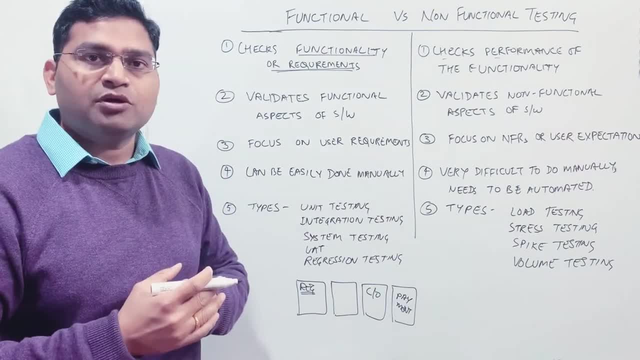 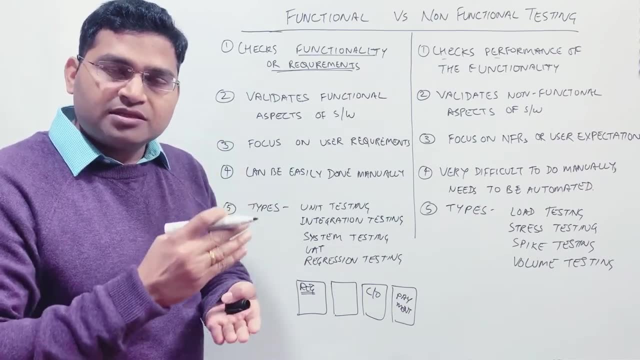 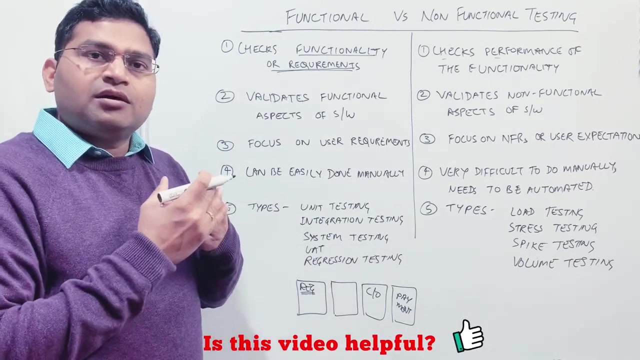 aspect of the same functionality: how much response time or what is the response time for actual user registration? how much time is the response time for the actual user registration time it takes, once user clicks on register button, to actually process the whole application and send the response back to the user, to actually register the user and send the response back to. 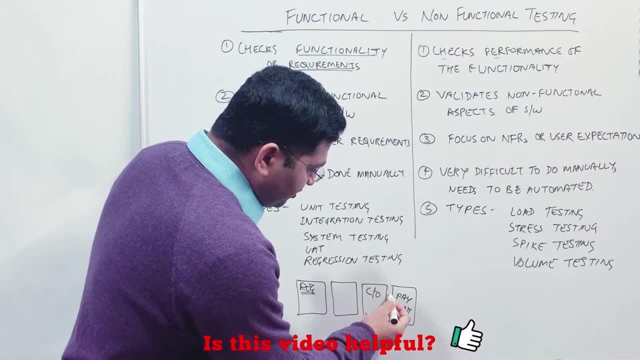 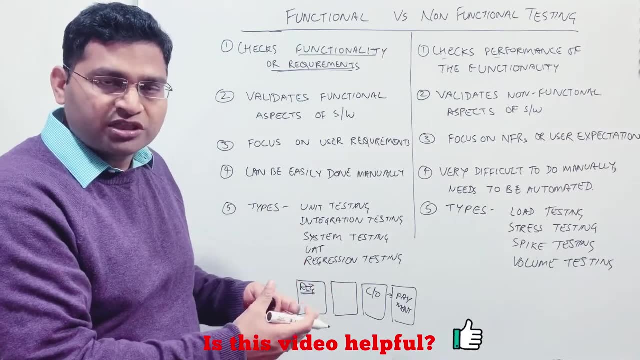 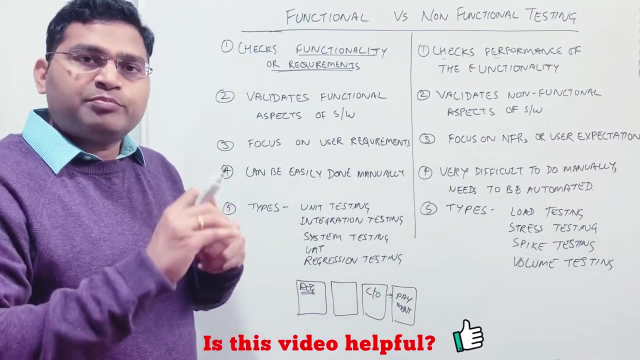 the user right. another example say, for example, payment. so i have added all the items in the card as a, as an end user or a person who wants to buy items on the e-commerce website, and then i clicked on payment. okay, so i provided my credit card details or debit card details and clicked on pay. 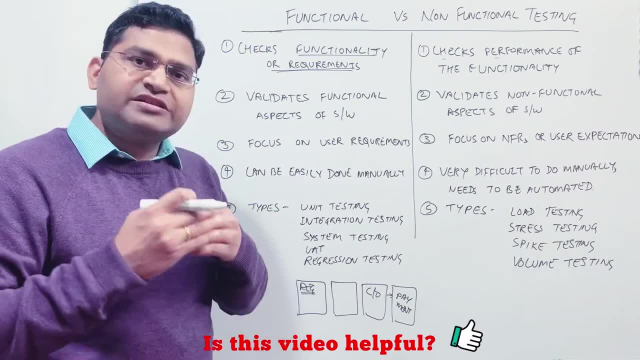 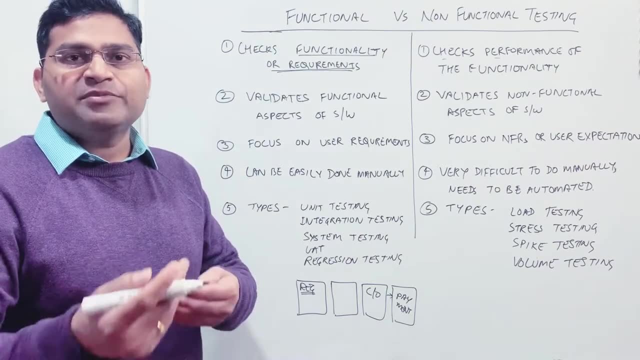 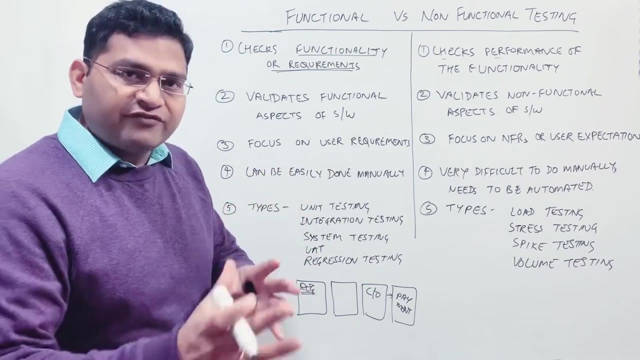 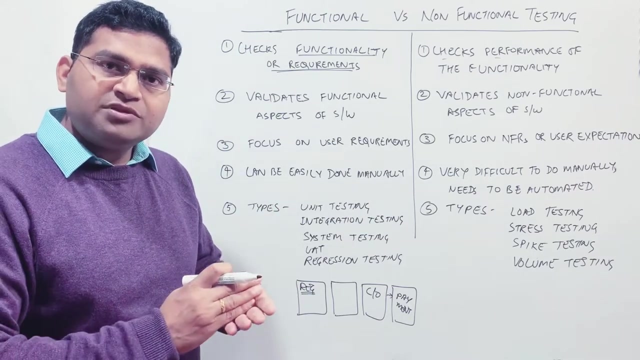 after clicking on pay, how much time it took to actually display me the message success, payment successful, and get me the order detail right or order number. so that is the non-functional aspect of the ordering functionality or the payment functionality right. so when i'm testing the functional aspect of the payment functionality, i'm 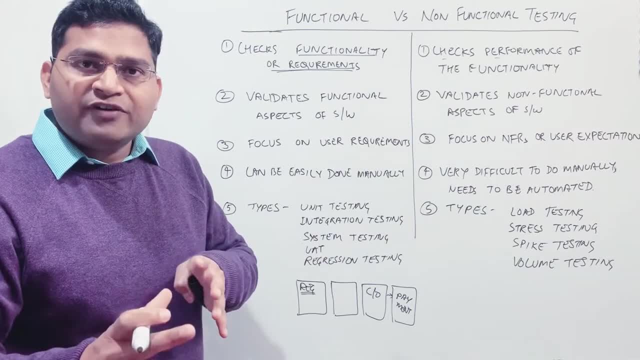 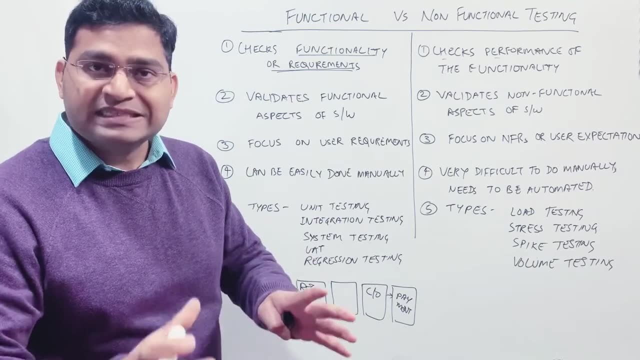 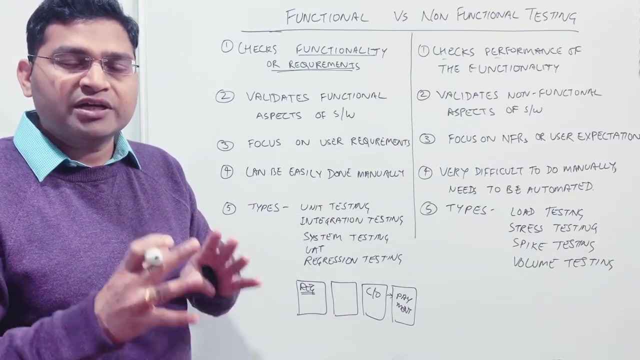 just worried about providing all the details and then verifying whether payment is successful or not. i'm not concerned whether the payment has been successful within 30 seconds or one minute or two minutes, but in the non-functional aspect or in non-functional testing i am worried about, or i 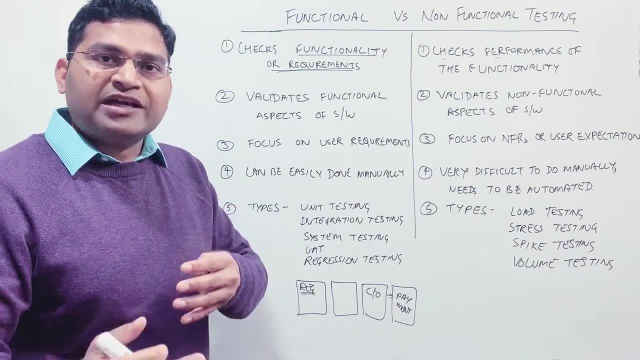 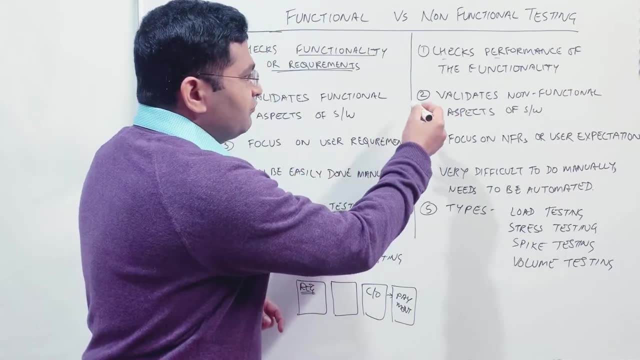 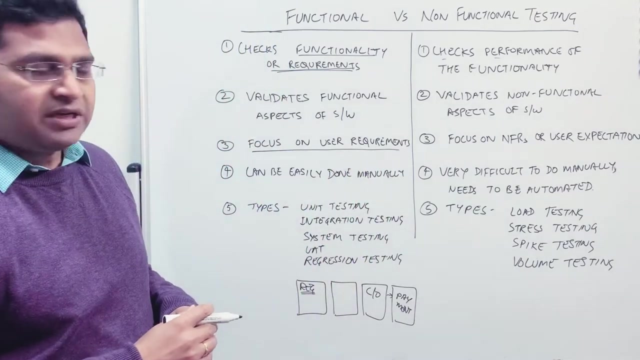 am concerned about how much time it takes to actually perform that particular operation. okay, so that is non-functional testing. second point: so it validates the non-functional aspects of the software. third point is basically focus on user requirements, right, so the most of the focus in on the user requirements. so, whatever requirement, functional requirement. 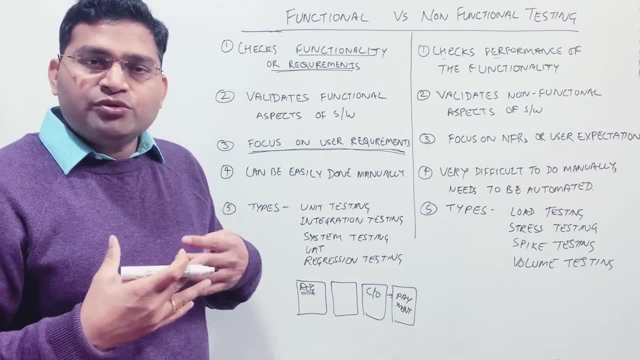 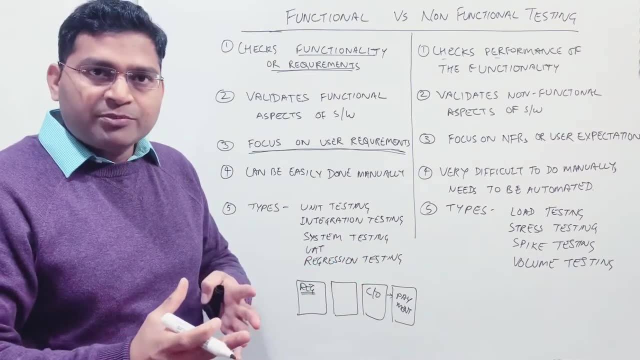 user will provide you. so, if i'm the end user or normal public is the end user, for example, in case of gmail or facebook social media website, we end users are, our normal public is the end user right? so, based on market research, there will be. you know some of the most important aspects of the software. 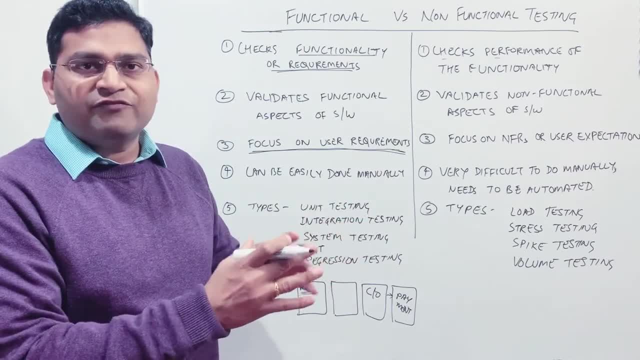 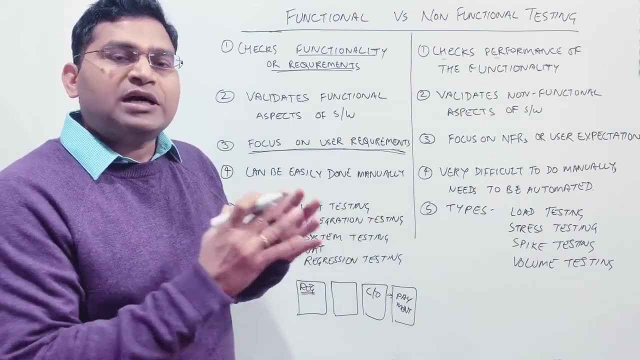 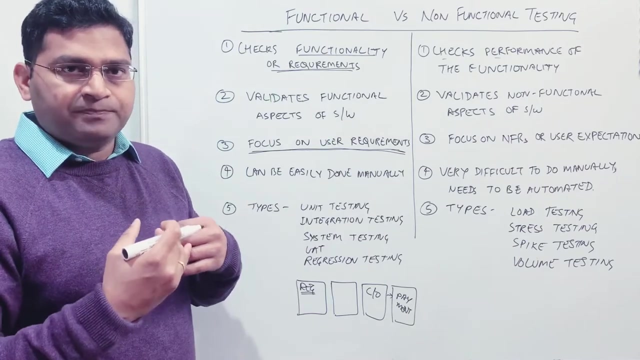 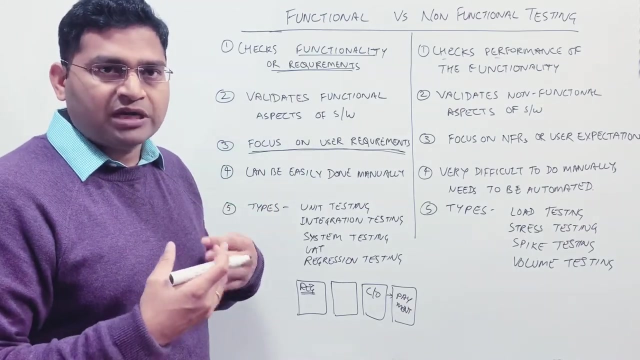 analysis done by the companies, and Facebook will implement those new functionalities. But if it is an organization who wants a software developed, then they will provide the requirements to the organization who is developing software for them. So in that case, if I am the organization who wants software to be developed, I am the customer. I'll provide. 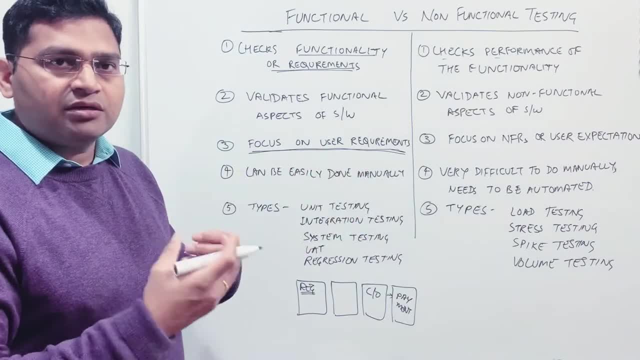 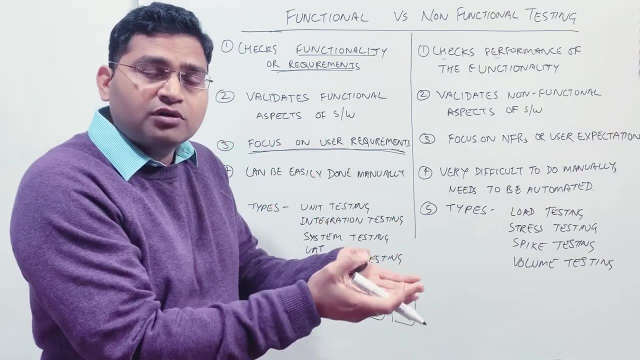 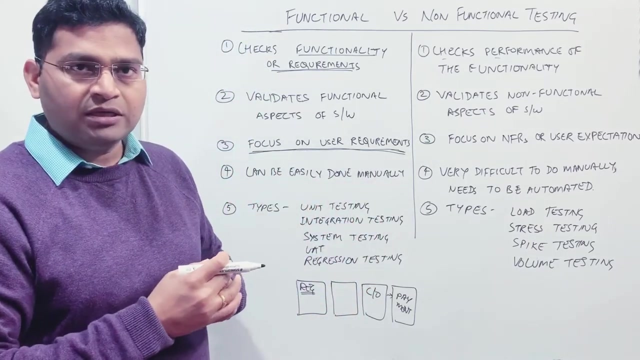 the requirement to the organization and they'll implement the software. for me, The focus on the functional testing is: whatever requirement I will provide for the software to be built. In case of e-commerce websites, for example, I want user registration using email. that's one of the requisites If I want to use registration using 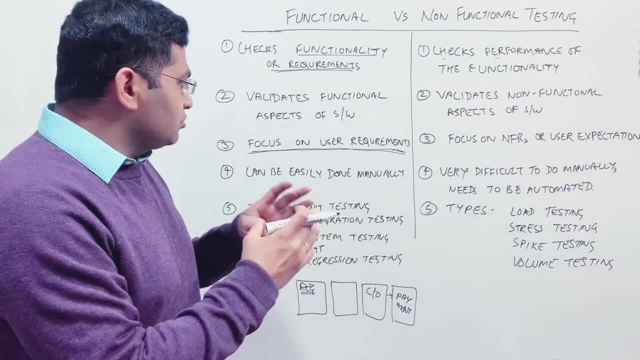 Facebook, Google account as well. that's another requirement. So if in the functional testing the organization will focus on the actual user requirement that it will send to the company, then they will implement the software for me. So the focus on the functional tests is whatever requirements I'll provide to the organization. 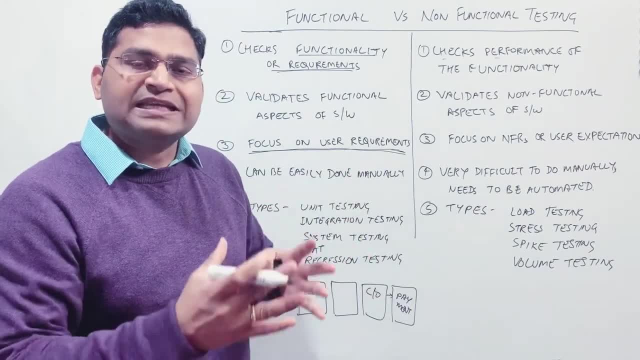 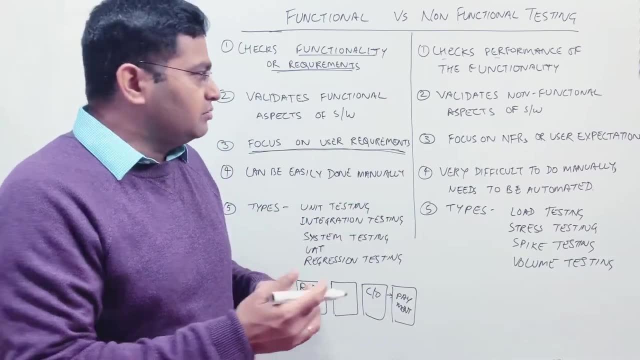 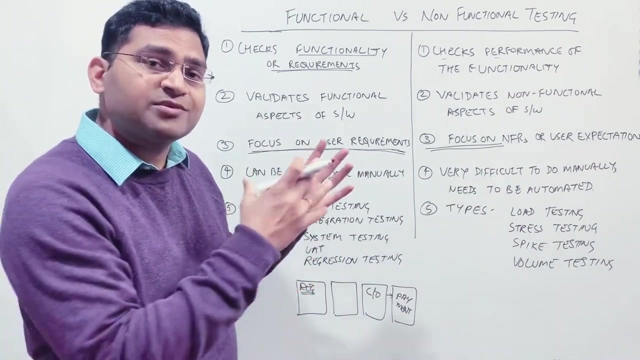 I'll provide. So whether those requirements or those functionalities are working, whether registration is actually working, they are not concerned about the performance of the registration Right. So the third point in the non-functional testing is it focuses on the non-functional requirement or user's expectation. Now NFRs, non-functional requirement and user expectation. 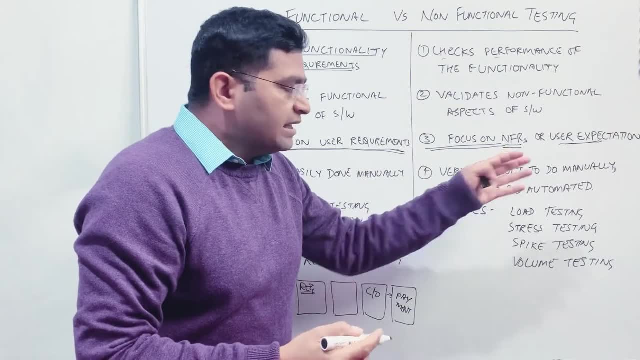 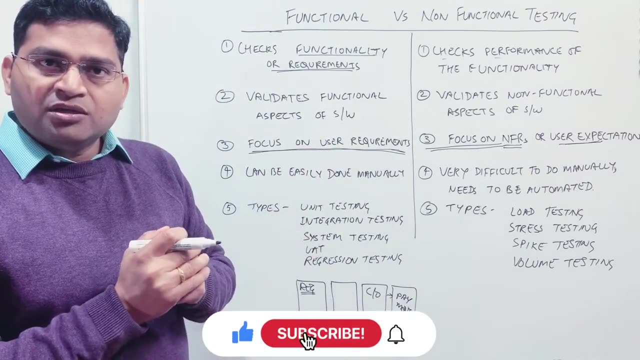 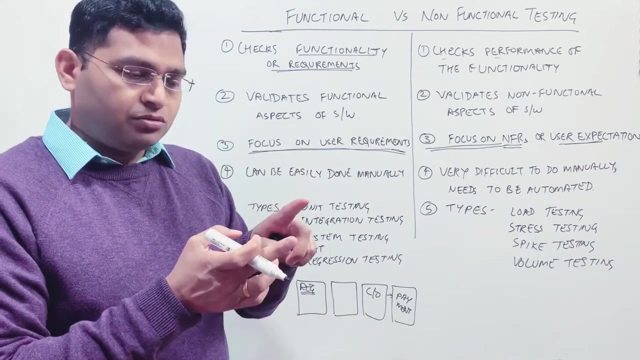 this is important to understand When we talk about NFR. so when I, as a customer, provide the requirement, I'll provide the functional requirement, user requirements. So, for example, registration using email, registration using Facebook account, registration using you know. 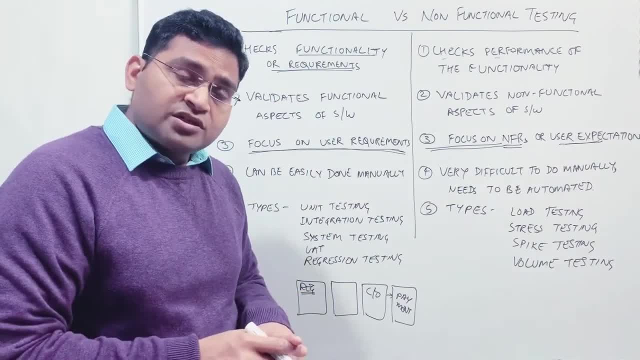 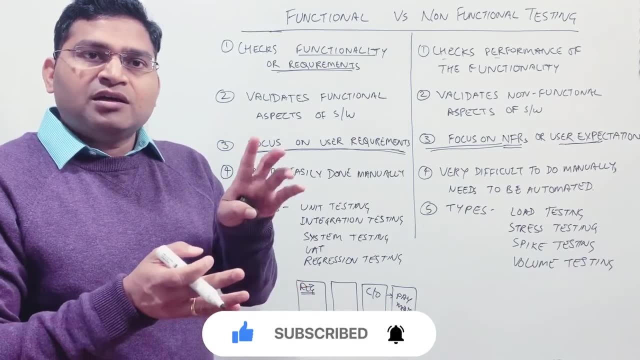 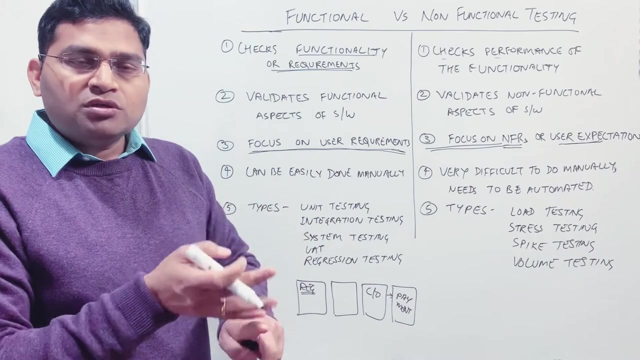 Google account, And then I'll also provide non-functional requirement for those requirements. So, for example, for registration, I'll mention to the customer that for up to 5,000 concurrent users on my e-commerce website, I want the response time of registration. 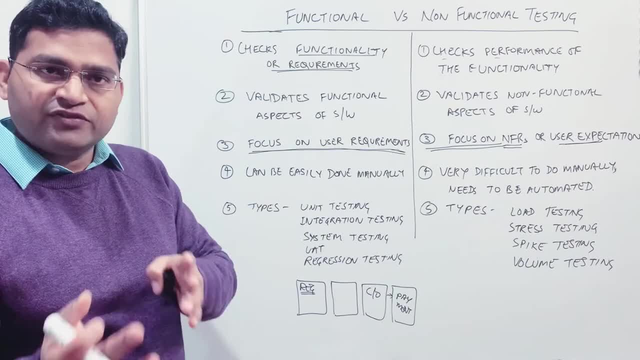 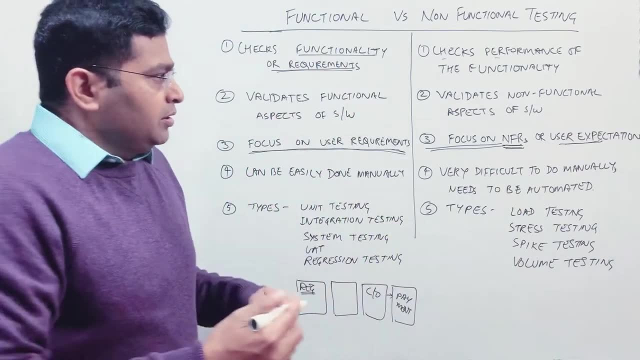 I want the registration functionality not to be more than five seconds. If that is the requirement or that is the non-functional aspect, then that is what non-functional requirement is. Now. user expectation is in the case. say, for example, I'm the normal public and 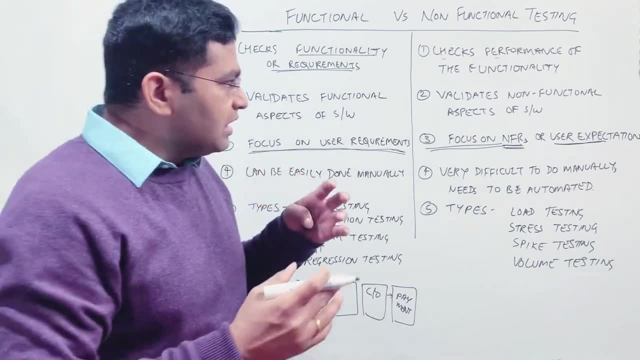 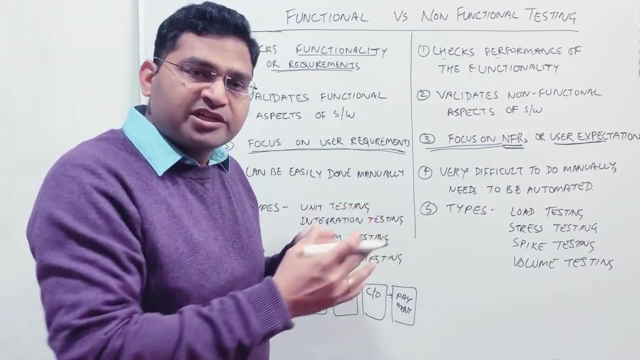 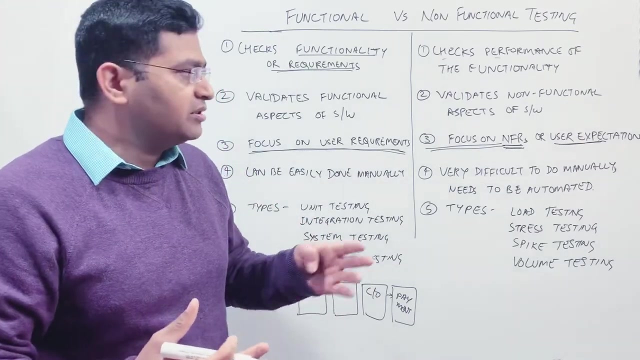 you know, or even if I'm the customer, So I expect the software to respond in particular, or the performance should be, you know, as per expectation. It shouldn't be like when I'm trying to register, It takes a minute to send me the response or register me as a user. That's not what. 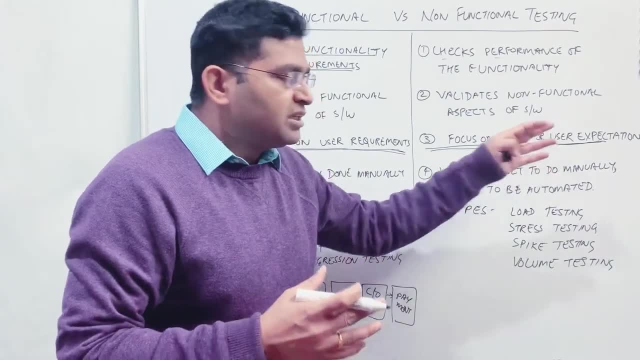 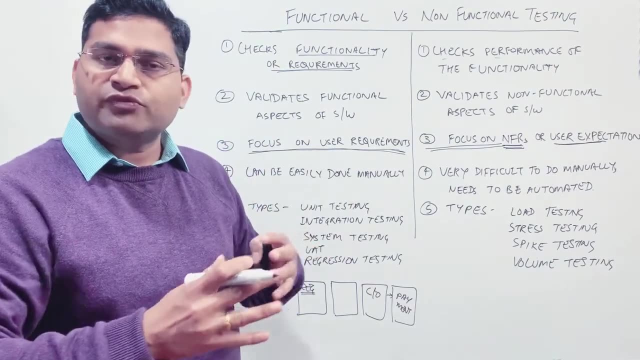 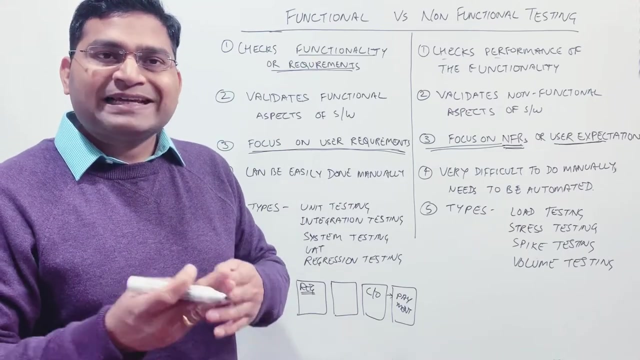 the usual user expectation is. But user expectation is more relevant when the functionality is being built by the end users, for example, users of Facebook right. So if I'm accessing Facebook, my user expectation is that within seconds, if I launch app, Facebook should. 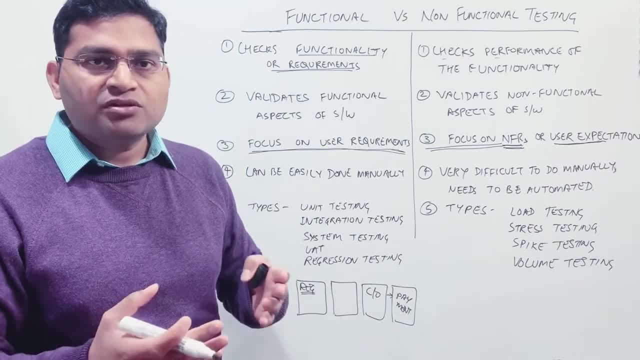 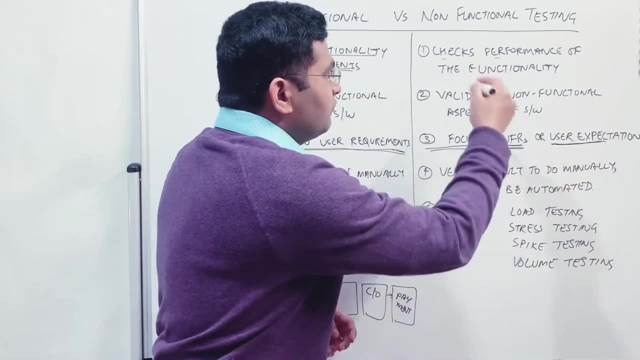 open for me. If it's taking 30 seconds or a minute to open the app, I should be able to log in, So that's why it is not fulfilling my expectation right. So in the non-functional requirement or non-functional testing, my core focus is on non-functional requirement. 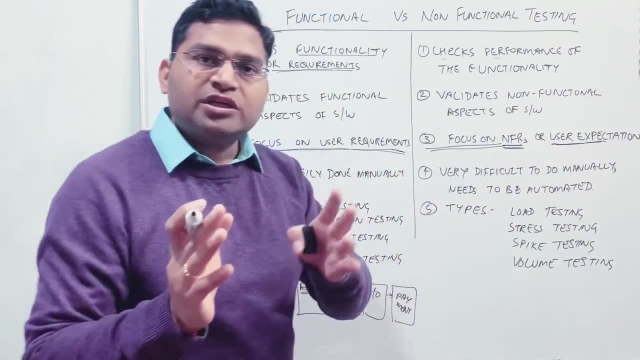 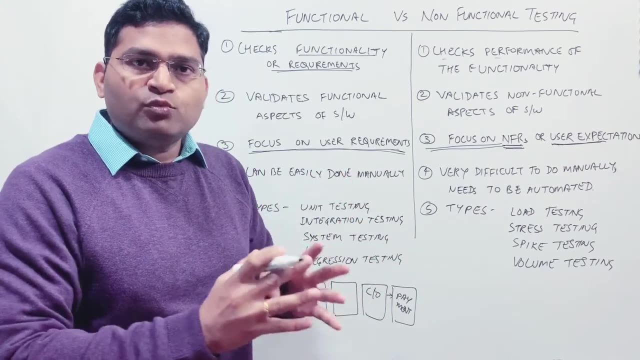 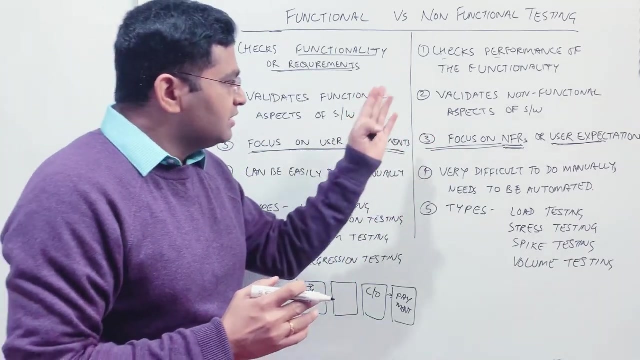 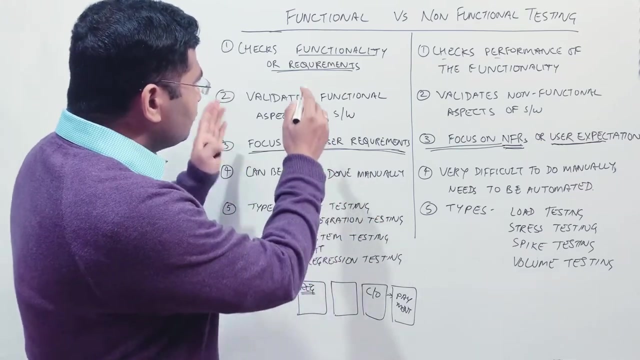 of the functionality or the requirement or the user expectation right. So in terms of user expectation, whether end user will be happy with the performance that we provide in the application for the application or not. So that's the non-functional testing versus functional testing. Then the point four is: can be easily done manually, So functional. 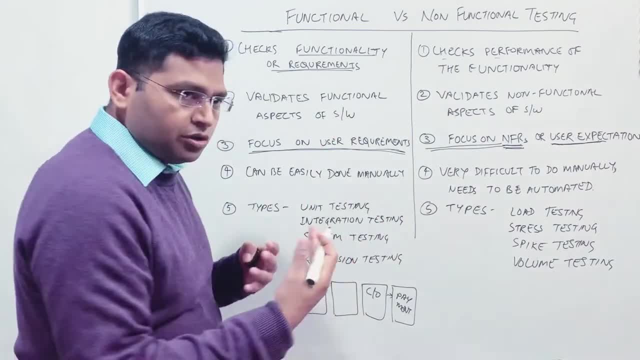 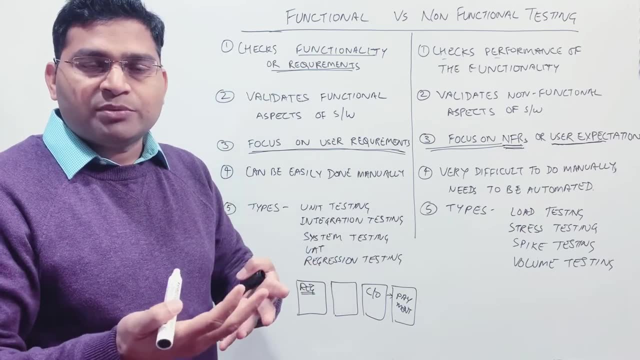 testing can be very easily done manually. So we can, you know, launch the e-commerce website, click on register button, provide the details. So all that is possible here. You can, you know, test e-commerce website in any of the browser or if there is an app. 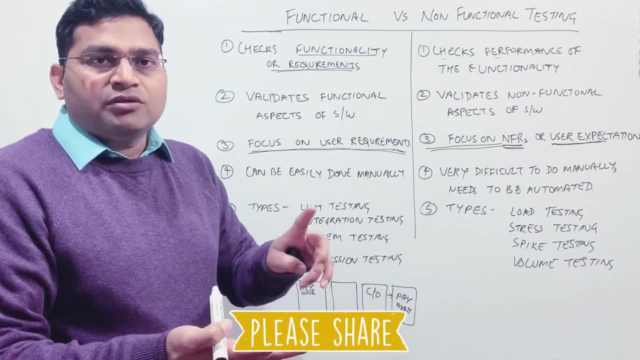 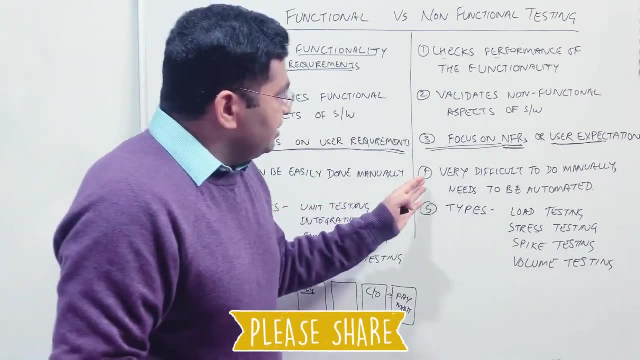 Android app or iOS app, you can quickly install it and launch the app manually and test it right. So you can do it manually as well as automated very easily. But in terms of non-functional testing, it is very, very difficult to do manually. Okay. 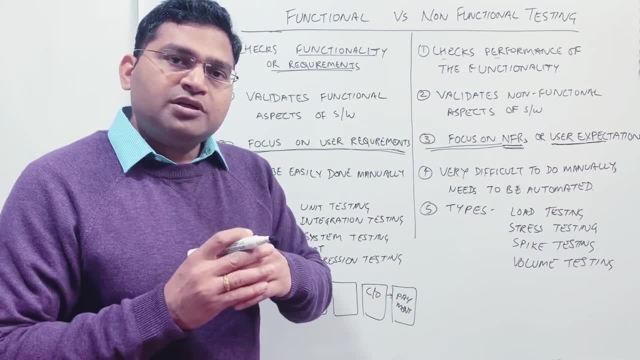 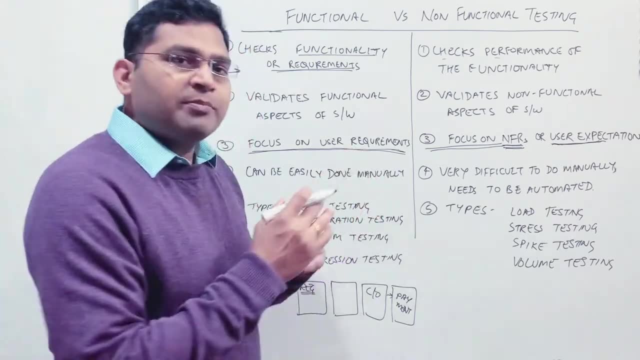 The reason is: say, for example, your customer requirement is that 5,000 concurrent users and the response time should be less than five seconds. So if you want to do it manually, you have to basically ask 5,000 people to log into the particular portal or access the. 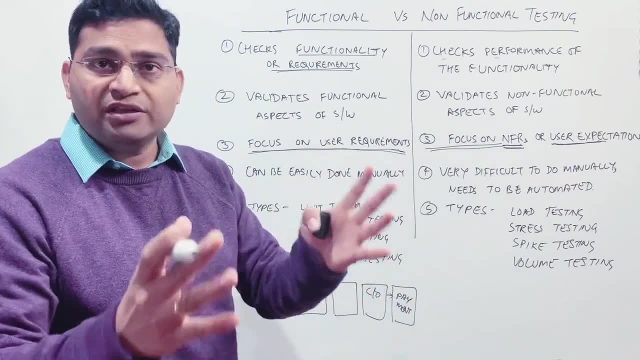 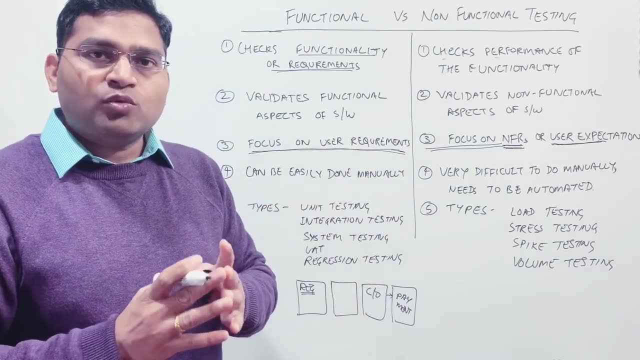 particular website at one particular time, which is very difficult to coordinate. And this is just. you know, like a, you know a small. you know like a, you know a small number. Your application might be required to respond well, for even you know a hundred. 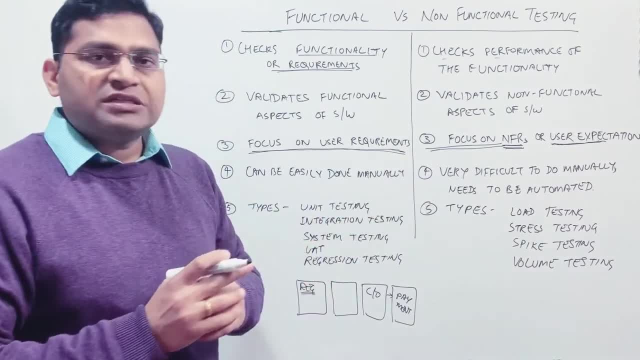 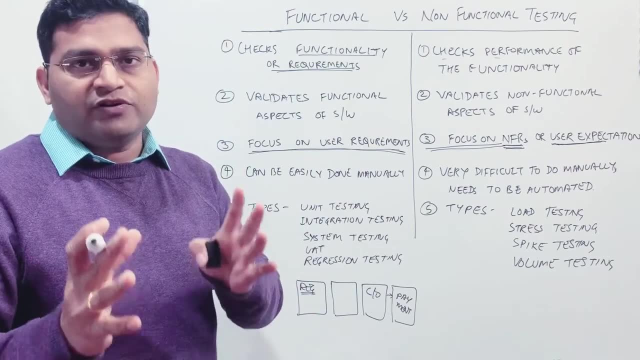 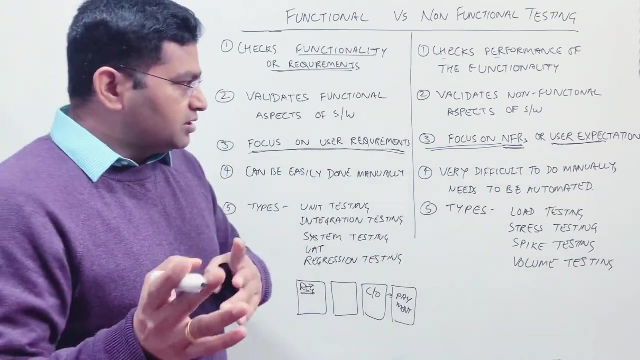 thousand users. So manually performing the non-functional testing is really not possible. It has to be automated. So there are tools available for non-functional testing that you can utilize for automation, And some of the tools are like: Loadrunner is one of the tools. NeoLoad is another tool. right, JMeter is a very, very popular open source tool. 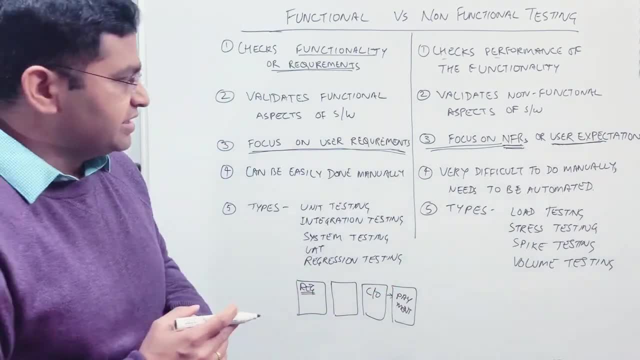 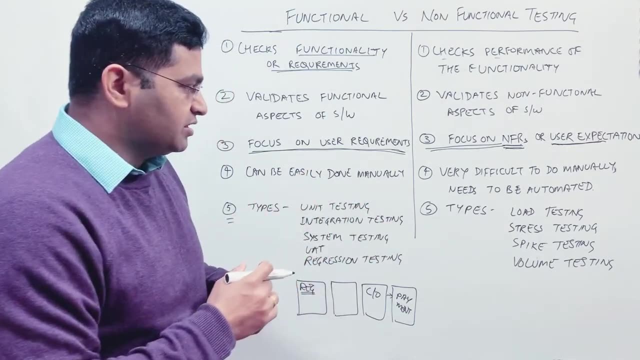 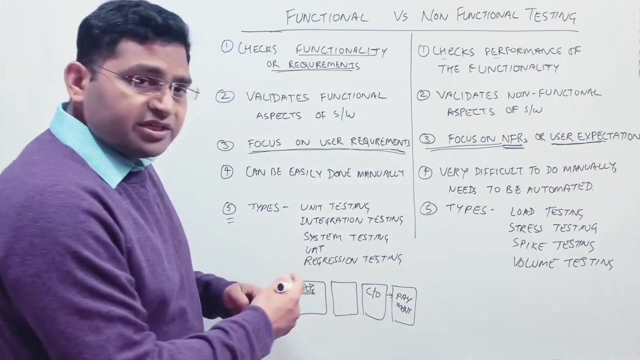 So all of those tools can be utilized for non-functional testing. The last point is around explaining the types of functional testing and types of non-functional testing. So in functional testing you have unit integration system, user acceptance testing, regression testing and there are many, many more types of testing in functional testing.